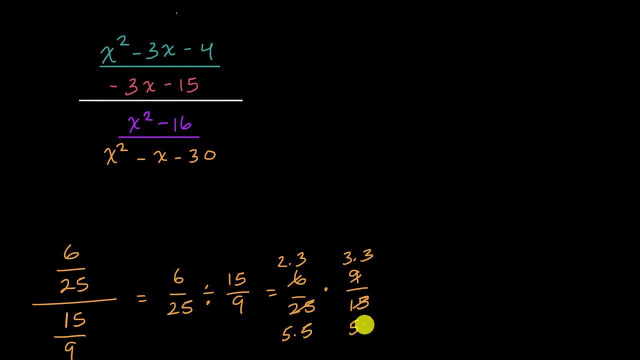 This is five times five, This is five times three. Let's see three in the numerator, three in the denominator, And actually that's about as far as we can get. So then we'll have two times three times three, which is going to be 18 in the numerator. 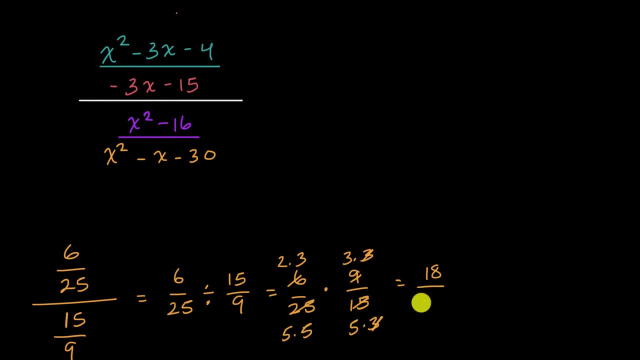 And then in the denominator we have five times five times five, which is 125.. So we're going to do the exact same thing up here, but there's one extra complication: We have to keep track of the x values. that would make us. 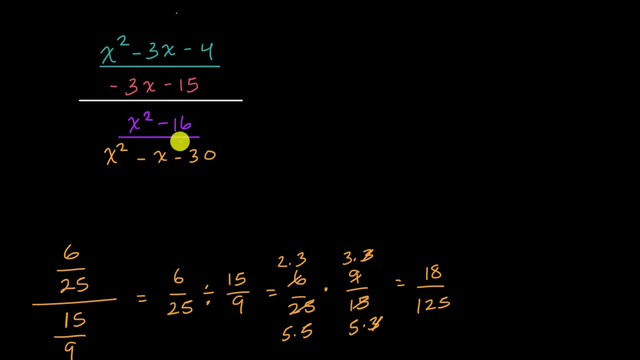 would make this expression undefined in any way, because as we reduce to lowest terms, we might lose that information. But if we lose that information, then we have changed the expression. So we have to keep track of how we are constraining this domain. 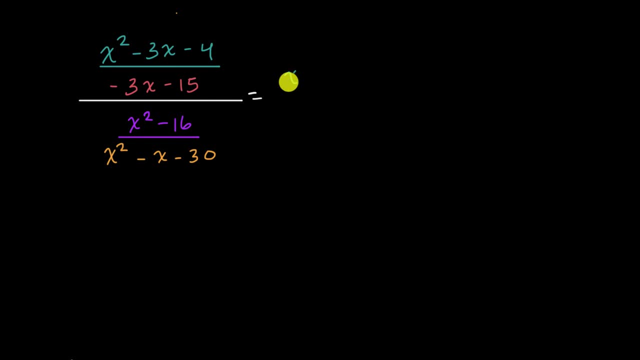 So first I can just rewrite this as x squared minus three, x minus four, all of that over negative three x minus 15.. And that's getting divided by divided by this business, x squared minus 16. over we have x squared minus x minus 30.. 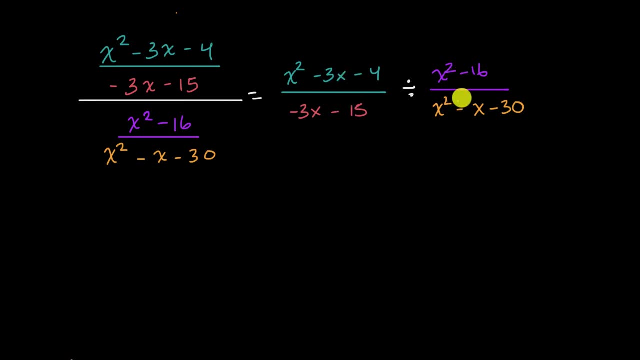 Now the next thing we can do is we can factor the various numerators and denominators and think about which x values could get us into trouble. So x squared minus three, x minus four, let's see negative one. let's see negative four times plus one. 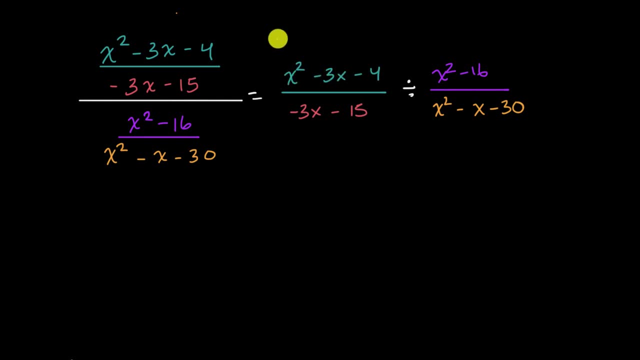 would be negative four, and then these would add up to negative three. So I can rewrite this as x minus four times x plus one. Rewrite it that way, And then I can rewrite what I have down here. I could factor out a negative three. 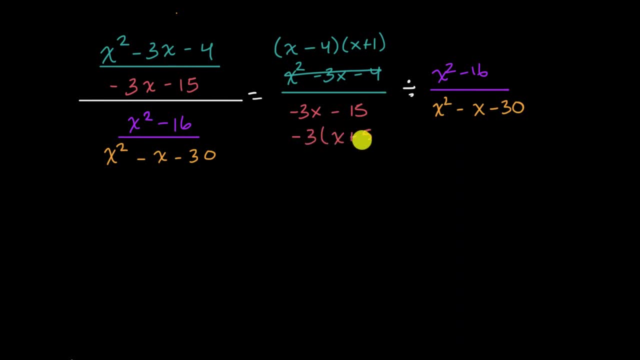 So I could write that as negative three times x plus five. And then I could write this one here: This is a difference of squares- is going to be x plus four times x minus four. And then, last but not least, this one over here: 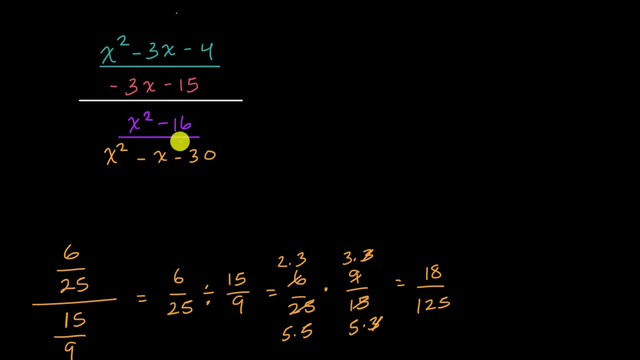 would make this expression undefined in any way, because as we reduce to lowest terms, we might lose that information. But if we lose that information, then we have changed the expression. So we have to keep track of how we are constraining this domain. 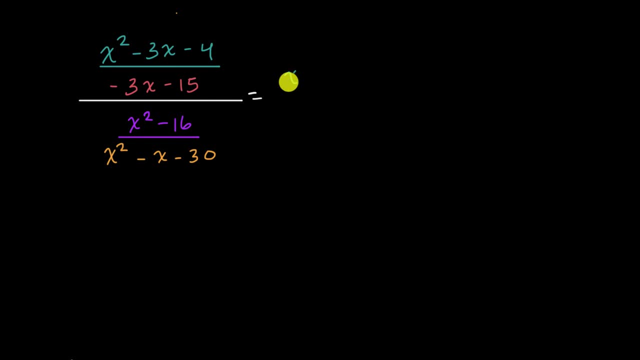 So first I can just rewrite this as x squared minus three, x minus four, all of that over negative three x minus 15.. And that's getting divided by divided by this business, x squared minus 16. over we have x squared minus x minus 30.. 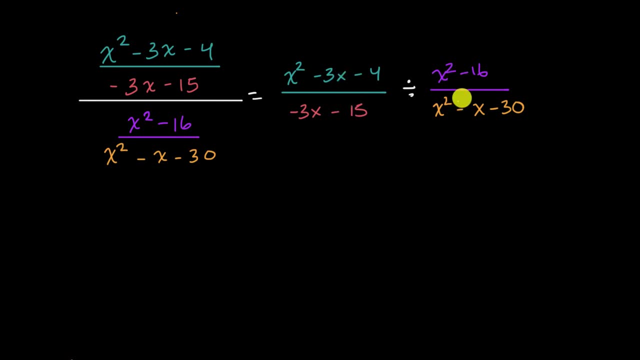 Now the next thing we can do is we can factor the various numerators and denominators and think about which x values could get us into trouble. So x squared minus three, x minus four, let's see negative one. let's see negative four times plus one would be negative four. 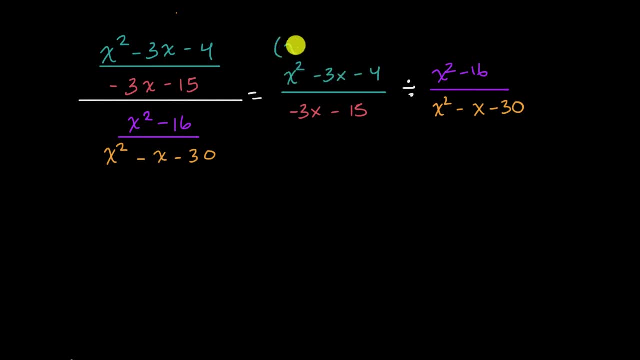 and then these would add up to negative three. So I can rewrite this as x minus four times x plus one. Rewrite it that way, And then I can rewrite what I have down here. I could factor out a negative three, So I could write that as negative three times x plus five. 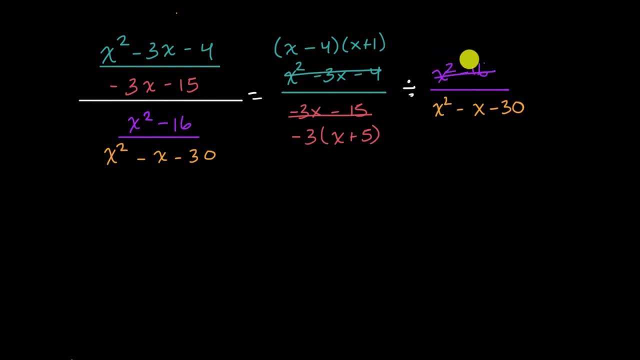 And then I could write this one here: This is a difference of squares- is going to be x plus four times x minus four. And then, last but not least, this one over here: let's see if I have a five and a six. 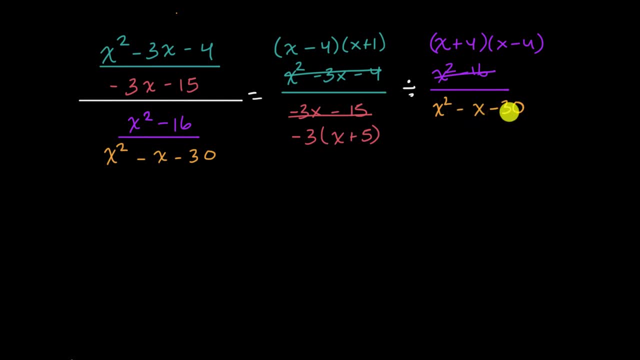 negative six plus five is negative one. negative six times five is negative 30. So this is going to be x minus six times x plus five. Now, before I go any further- and the reason why I factored at that point is now we can think about what x values. 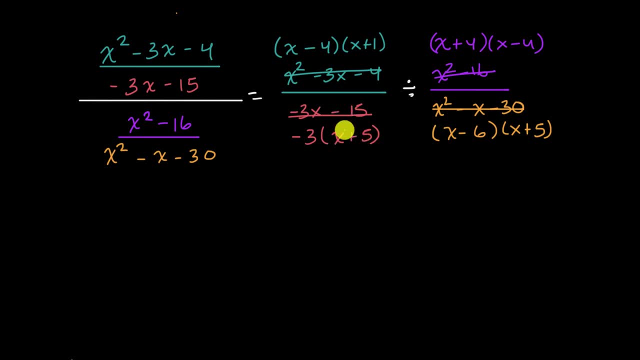 will get us in trouble. We know that any x values that make any of the denominators equal to zero, that would be undefined. So we want to constrain our domain in that way. So we know, for example, that x cannot be equal to negative five. 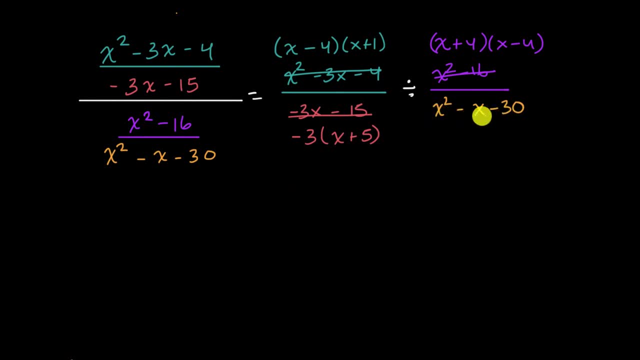 let's see if I have a five and a six negative. six plus five is negative. one negative. six times five is negative 30. So this is going to be x minus six times x plus five. Now, before I go any further, 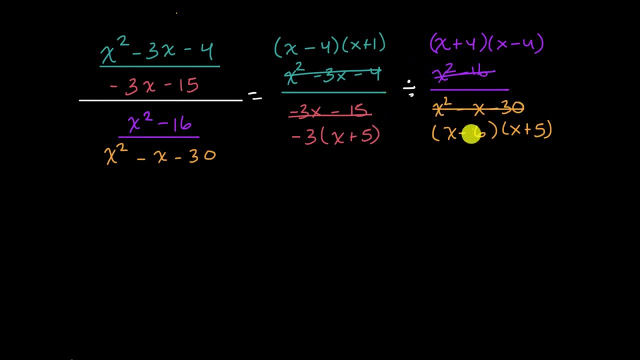 and the reason why I factored at that point is now we can think about what x values will get us in trouble. We know that any x values that make any of the denominators equal to zero, that would be undefined. So we want to constrain our domain in that way. 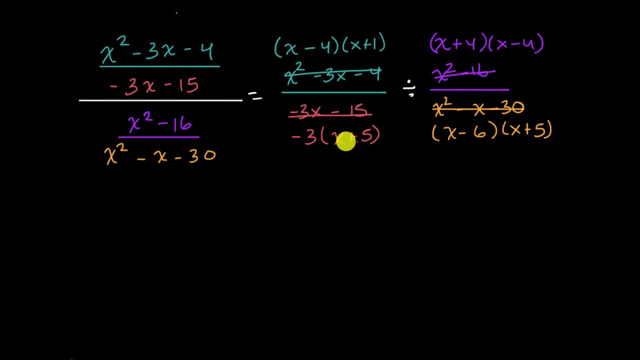 So we know, for example, that x cannot be equal to negative five. That would make this denominator equal to zero. Let me write that here. So x cannot be equal to negative five. We also know that x cannot be equal to six. 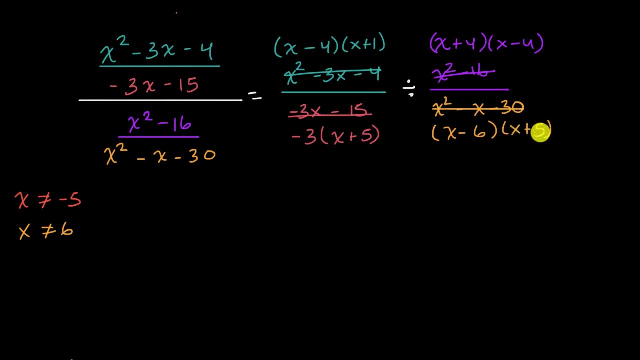 x cannot be equal to six, And this would also tell us that x cannot be equal to negative five. Let me write that again, But we're not done. So we've figured out the x values that make these denominators equal to zero. 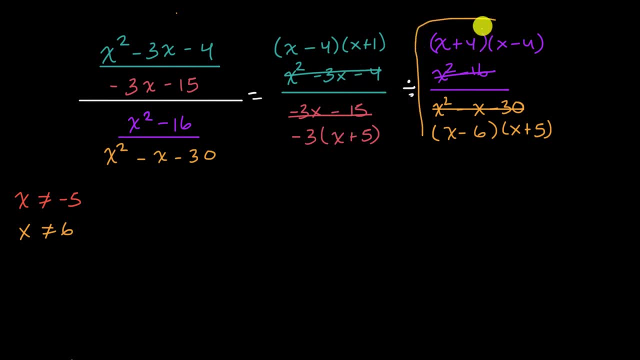 But remember, we're also dividing by this entire expression here. So anything that would make the entire expression equal to zero would also be a problem, because you can't divide by zero. So anything that would make this numerator equal to zero, which was this numerator right over here. 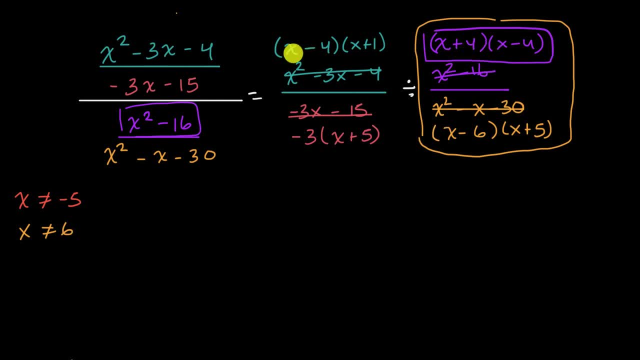 would make us also divide by zero. So we have to constrain there, Not this numerator here. That one's fine, That one could be equal to zero, That's complete. We can't divide zero by other things. So let's see. 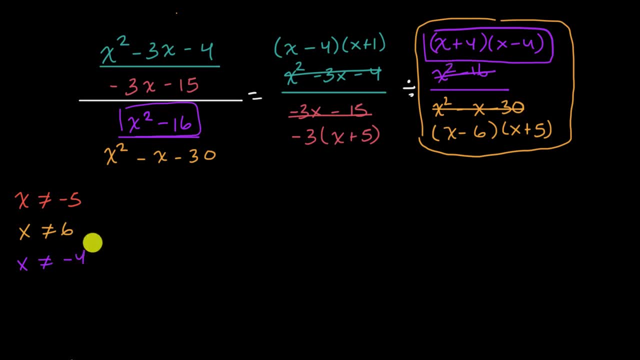 We could see that x cannot be equal to negative four, And actually x cannot be equal to positive four. So now we've fully constrained our domain And now we can proceed. So let me box this off right over here, And then we continue. 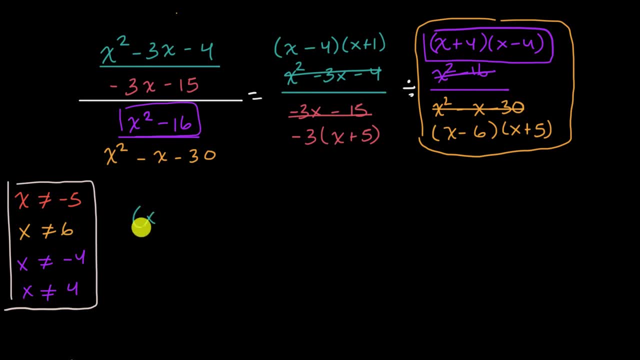 I can rewrite all of this. So we're going to have x minus four times x plus one, all of that over negative three. And then we have x minus four times x plus five. And now I'm just going to, instead of divide by this: 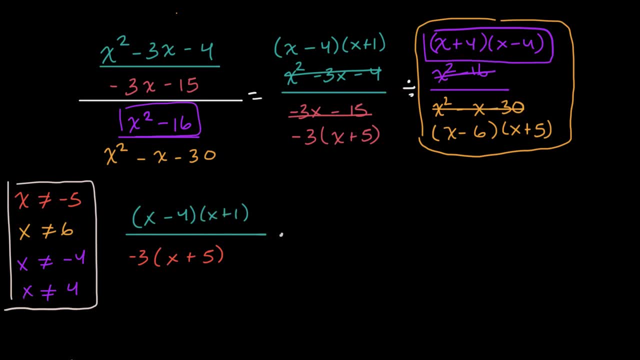 I'm going to multiply by the reciprocal. So this is going to be times, and I'm just going to take the reciprocal x minus six times x plus five. All of that over, we have x plus four times x minus four And once again our domain is constrained in this way. 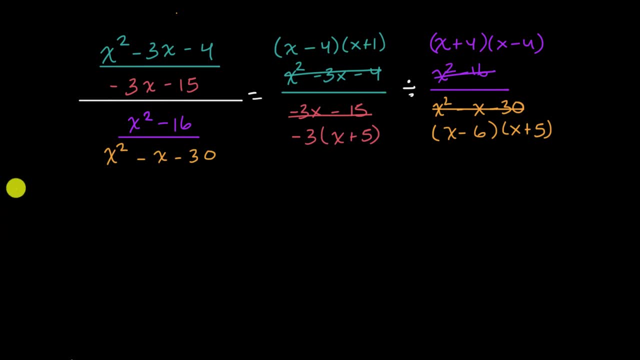 That would make this denominator equal to zero. Let me write that here. So x cannot be equal to negative five. We also know that x cannot be equal to six. x cannot be equal to six, And this would also tell us that x cannot be equal to negative five. 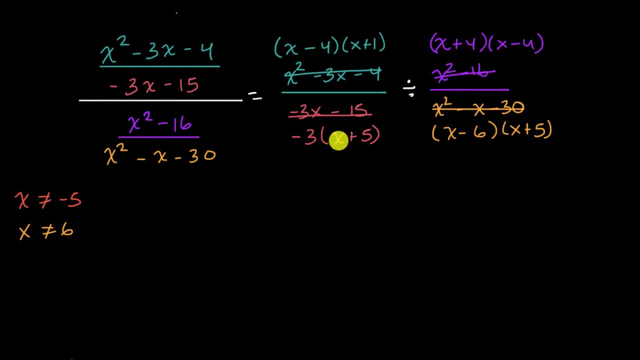 So I don't have to rewrite that. Let me rewrite that again, But we're not done. So we've figured out the x values that make these denominators equal to zero, But remember we're also dividing by this entire expression here. 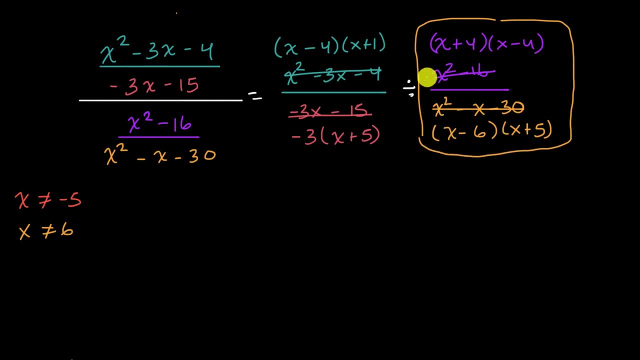 So anything that would make the entire expression equal to zero would also be a problem, because you can't divide by zero. So anything that would make this numerator equal to zero, which was this numerator right over here, would make us also divide by zero. 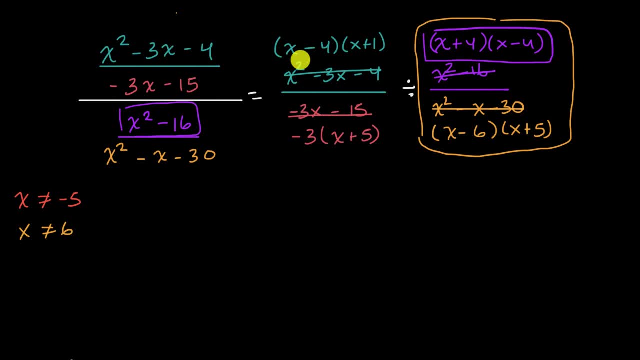 So we have to constrain there, Not this numerator here. That one's fine, That one could be equal to zero, That's complete. We can't divide zero by other things. So let's see, We could see that x cannot be equal to negative four. 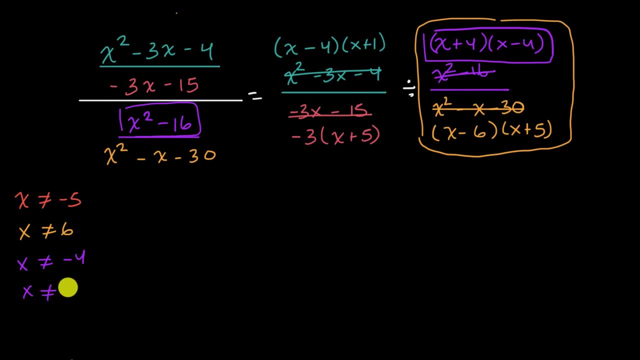 And actually x cannot be equal to positive four. So now we've fully constrained our domain And now we can proceed. So let me box this off right over here And then we continue. I can rewrite all of this. So we're going to have x minus four times x plus one. 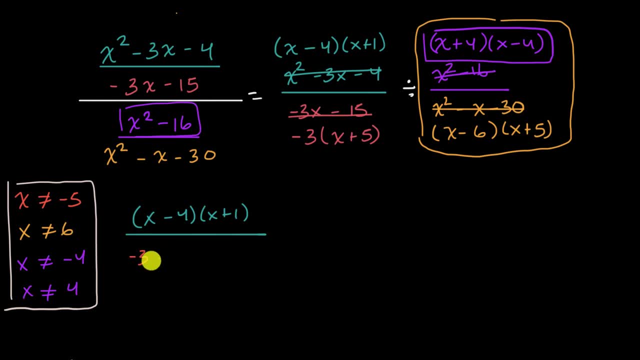 all of that over negative three, And then we have x minus four times x plus five, And now I'm just going to, instead of divide by this, I'm going to multiply by the reciprocal. So this is going to be times and I'm just going to take the reciprocal. 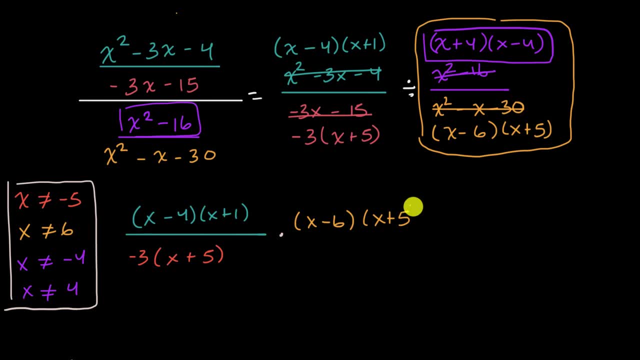 x minus six times x plus five. All of that over we have x plus four times x minus four, And once again our domain is constrained in this way. But we see we have an x minus four in the numerator, now x minus four in the denominator. 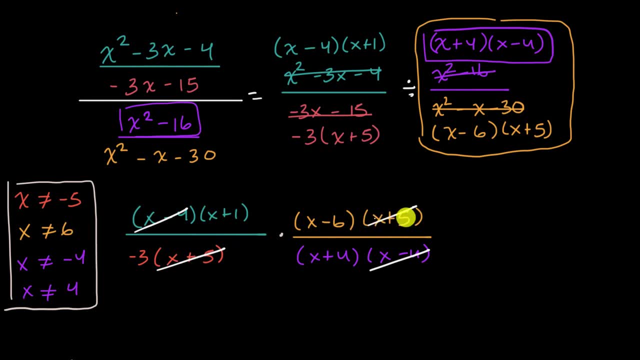 x plus five in the denominator, x plus five in the numerator, And now we can say that this is going to be equal to x plus one times x minus six. all of that over negative three, negative three times x plus four. x plus four.